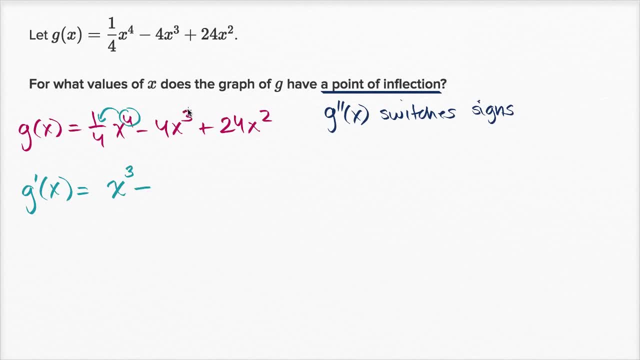 So four to the third power minus three times four is 12, x to the three minus one power, or x to the second power plus two times 24, or 48,, x to the two minus one or x to the first power. 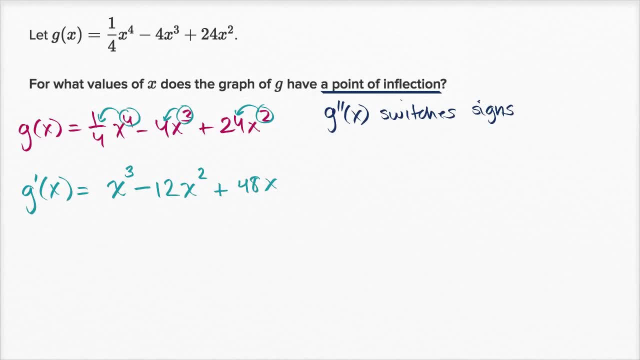 I could just write that as x. So there you have it. I have our first derivative. Now we wanna find our second derivative. We know that g prime prime of x, is just the derivative of the first derivative with respect to x, And so more of the power rule. 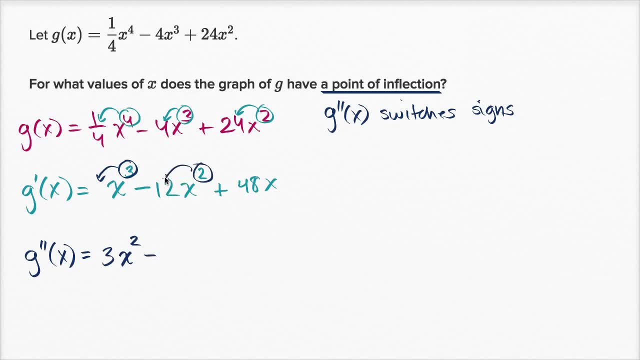 three x squared minus 24 x to the first, or just 24 x plus 48.. So let's think about where this switches signs. And this is a continuous function that's going to be defined for all x's, so the only potential candidates of where it could switch. 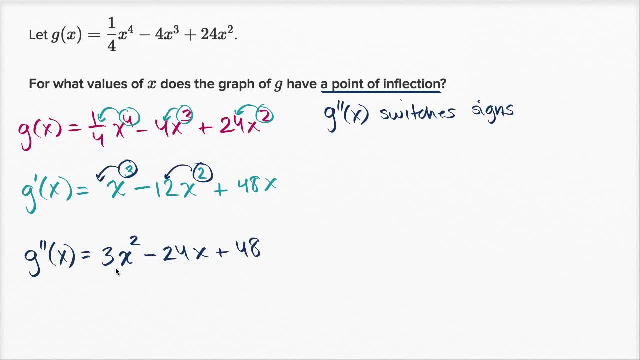 then this thing equals zero. So let's see where it equals zero. So let's set that equal to zero. Three x squared minus 24 x plus 48 is equal to zero. Let's see, everything is divisible by three. so let's divide everything by three. 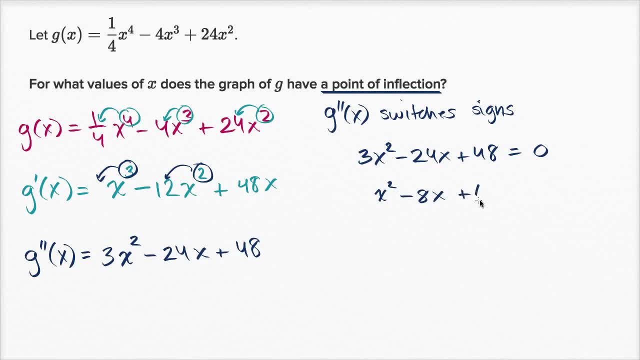 So you get x squared minus eight, x plus 16, plus 16 is equal to zero. And let's see, can I factor this? Okay, this would be x minus four times x minus four, Or you could just view this as x minus four squared. 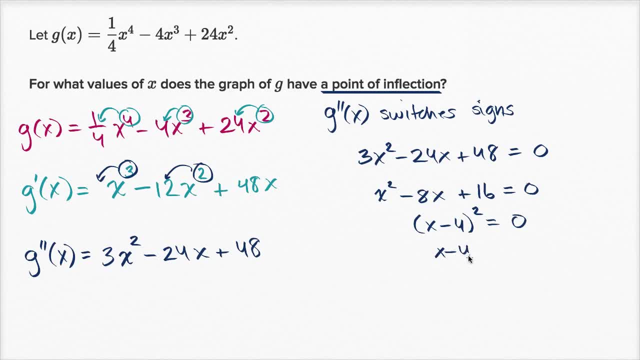 is equal to zero, or x minus four is equal to zero, or where x equals four. So g, prime prime of four, is equal to zero. So let's see what's happening on either side of that. Let's see if g, if we're actually switching signs or not. 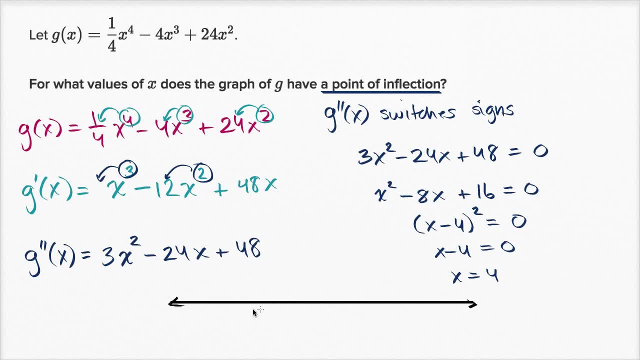 So let me draw a number line here, And so this is so. this is two, three, four, five, and I could keep going, And so we know that something interesting is happening right over here. G prime prime of four is equal to zero. 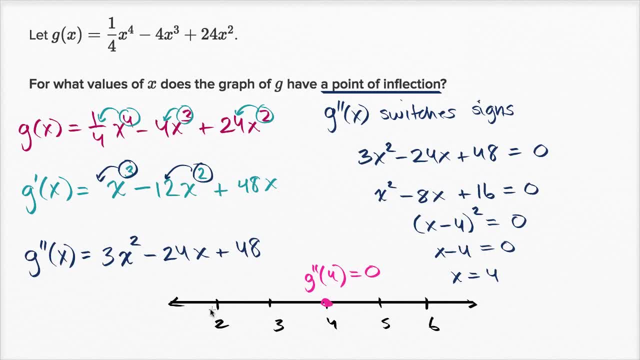 g prime prime of four is equal to zero. So let's think about what the second derivative is when we are less than four. And so actually, let me just try g prime prime of zero, since that'll be easy to evaluate g prime prime of zero. well, it's just going. 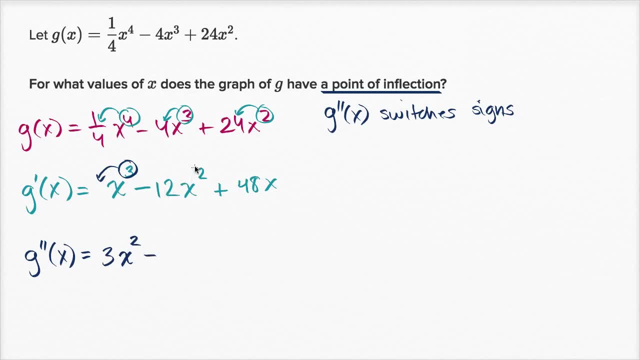 three x squared minus 24, x to the first, or just 24x plus 48.. So let's think about where this switches sides, And this is: this is a continuous function that's gonna be defined for all xs, So the only potential candidates. 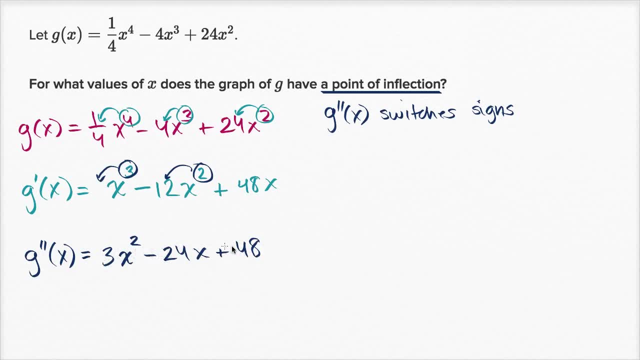 of where it could switch sides are when this thing is, this thing equals zero. So let's see where it equals zero. So let's set that equal to zero. Three x squared minus 24x plus 48 is equal to zero. Let's see, everything is divisible by three. 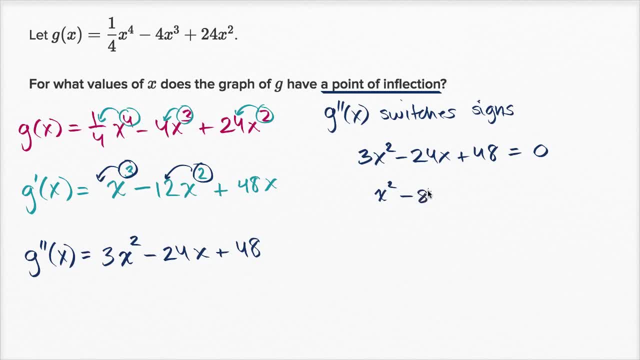 so let's divide everything by three, So you get x squared minus eight, x plus 16, plus 16 is equal to zero. And let's see, can I factor this? Okay, this would be x minus four times x minus four. 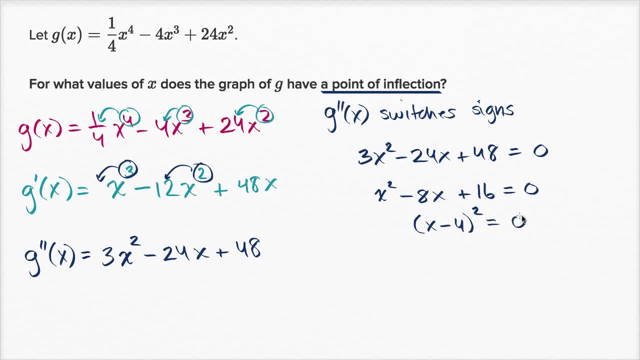 Or you could just view this as x minus four, squared, is equal to zero, Or x minus four is equal to zero, So, or where x equals four, So g prime prime of four is equal to zero, So let's see what's happening on either side of that. 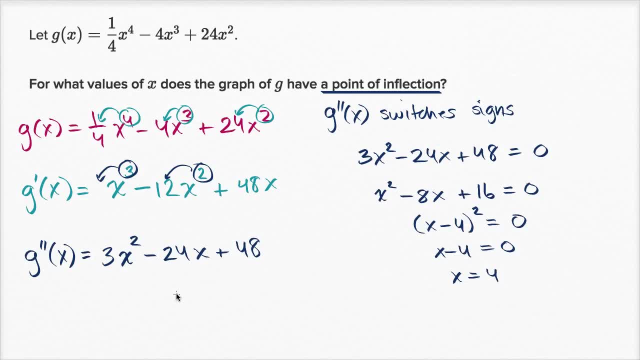 Let's see if g, if we're actually, if we're actually switching signs or not. So let me draw a number line here, And so this is. So this is two, three, four, five, and I could keep going, And so we know that something interesting. 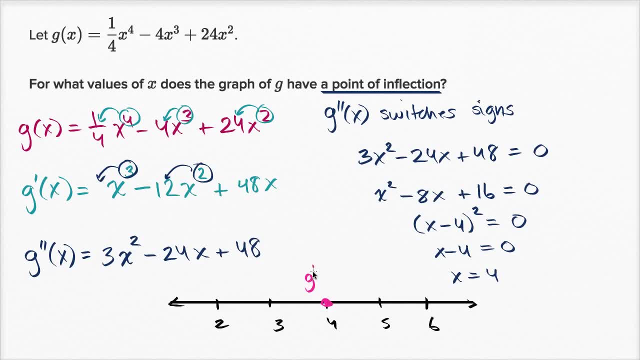 is happening right over here. G prime prime of four is equal to zero. G prime prime of four is equal to zero. So let's think about what the second derivative is when we are less than four. And so actually let me just try g prime prime of zero. 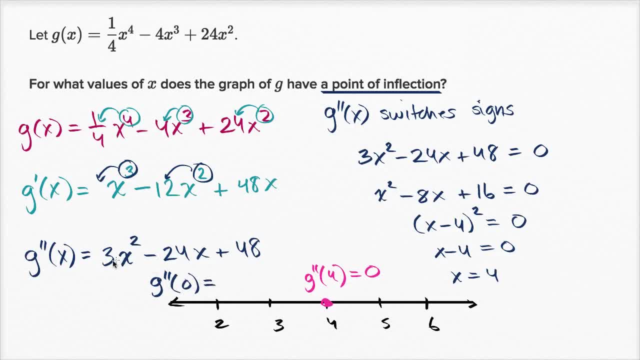 since that'll be easy to evaluate G prime, prime of zero. well, it's just going to be. it's going to be equal to 48. So when we are less than four, our second derivative, g prime, the second derivative, is greater than zero. 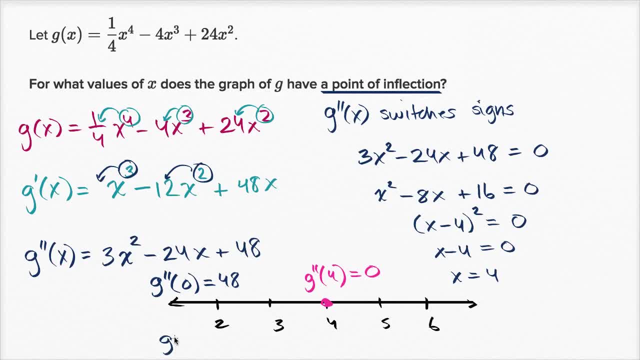 is going to be equal to 48. So when we are less than four, our second derivative, g prime, the second derivative, is greater than zero. So we're actually going to be concave upwards over this interval to the left of four. 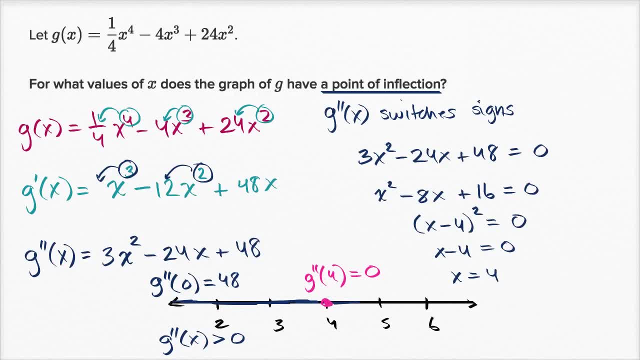 Now let's think about to the right of four. Two: this is a different color, So what about to the right of four? And so let me just evaluate. this would be an easy thing to evaluate. Well, I could evaluate g prime of. 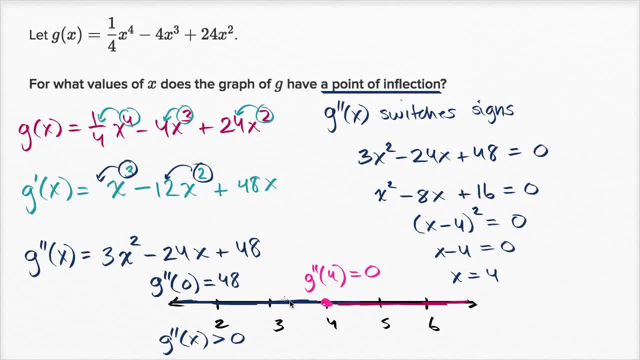 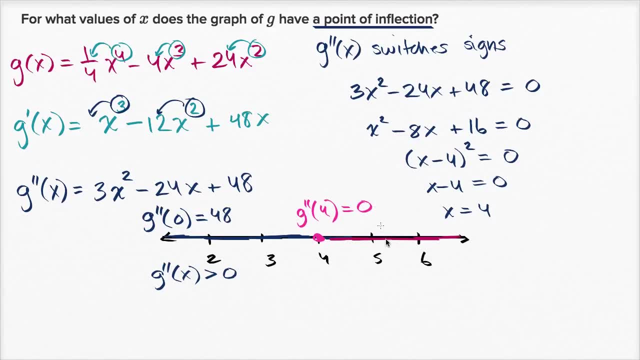 well, why not do g prime prime, I should say of 10.. So g, I'll do it right over here. Well, I'm running a little bit out of space, so I'll just scroll down. So g prime prime of 10 is going to be equal. 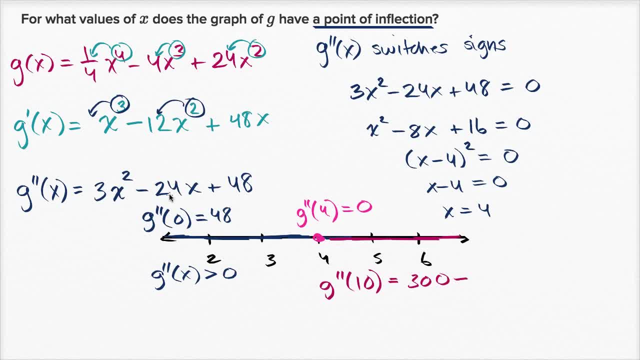 to three times 10 squared. So it's 300 minus 24 times 10.. So minus 240 plus 48.. So let's see this is 60.. This is so 300 minus 240 is 60 plus 48.. 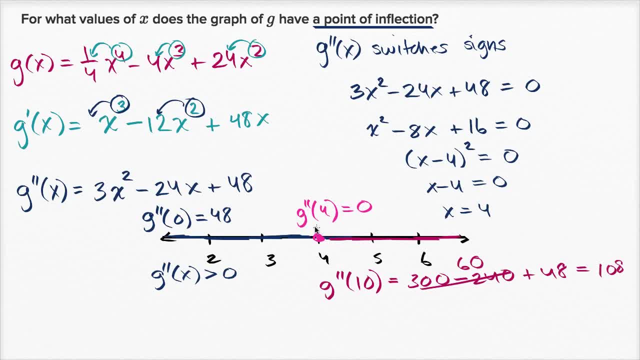 So this is equal to 108.. So it's still positive. So on either side of four, g prime, prime of x is greater than zero. So even though the second derivative at x equals four, is equal to zero, on either side we are concave upwards. 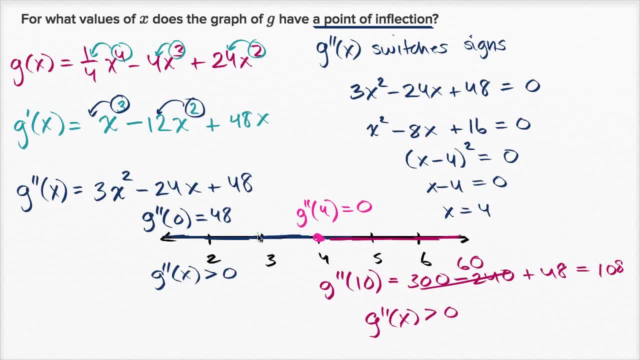 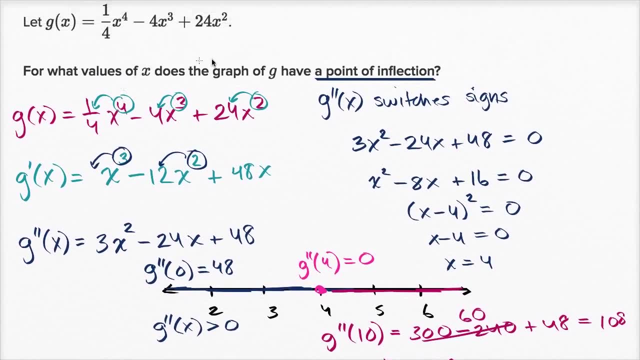 On either side. the second derivative is positive And so- and that was the only potential candidate, So there are no values of x for which g has a point of inflection. X equals four would have been a value of x at which g had a point of inflection. 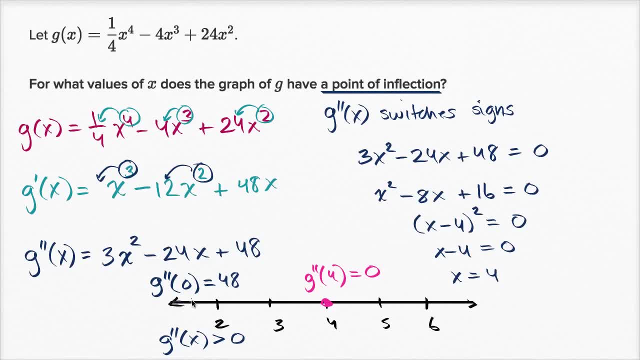 So we're actually going to be concave upwards over this interval to the left of four. Now let's think about to the right of four. Two, this is a different color, So what about to the right of four? And so let me just evaluate. 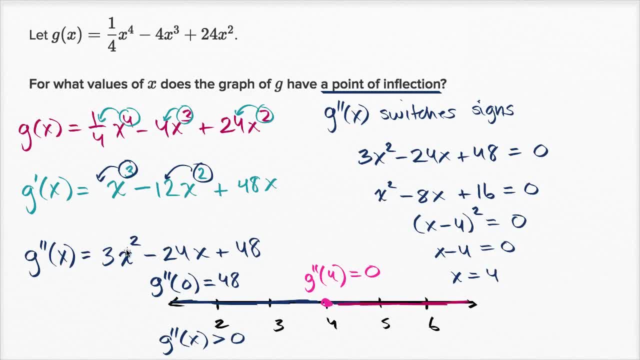 what would be an easy thing to evaluate. Well, I could evaluate g prime of. well, why not do g? or the second derivative, g prime, prime, I should say, of 10.. So g, I'll do it right over here. 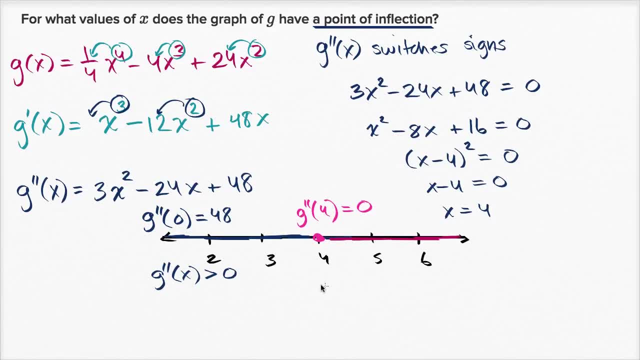 Let me do the. well, I'm running a little bit out of space so I'll just scroll down. So g prime prime of 10 is going to be equal to three times 10 squared. So it's 300 minus 24 times 10.. 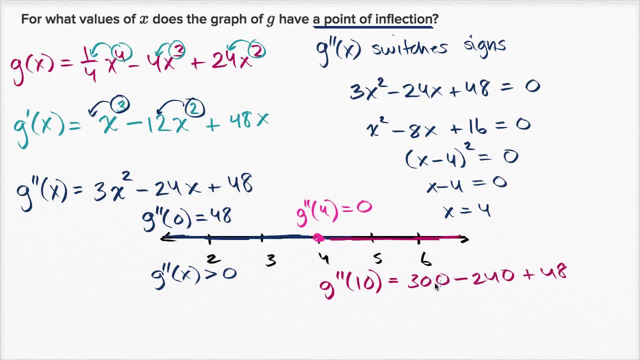 So minus 240 plus 48. So let's see, At 60, this is so 300 minus 240 is 60, plus 48. So this is equal to 108.. So it's still positive. So on either side of four g prime, prime of x. 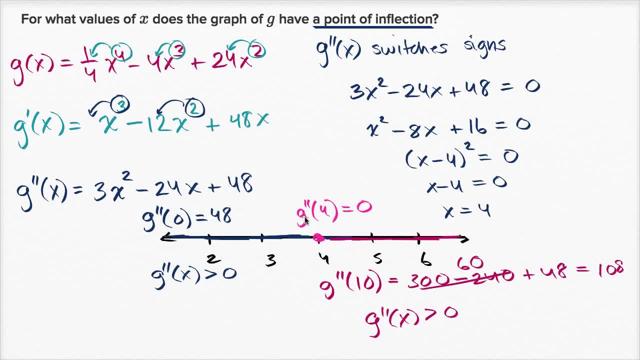 is greater than zero. So even though the second derivative at x equals four, is equal to zero on either side, we are concave upwards. On either side the second derivative is positive, And so that was the only potential candidate. So there are no values of x. 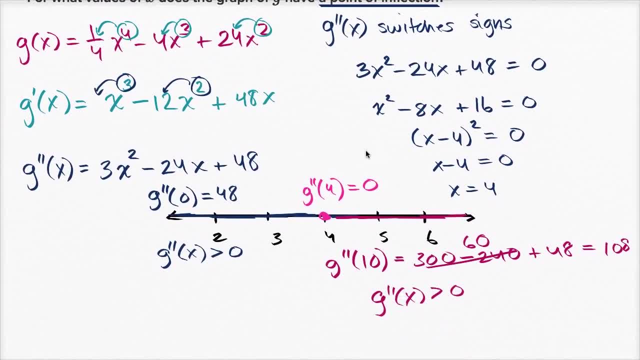 for which g has a point of inflection. X equals four would have been a value of x at which g had a point of inflection. if we switch, if the second derivative switched signs here, If it went from positive to negative or negative to positive. 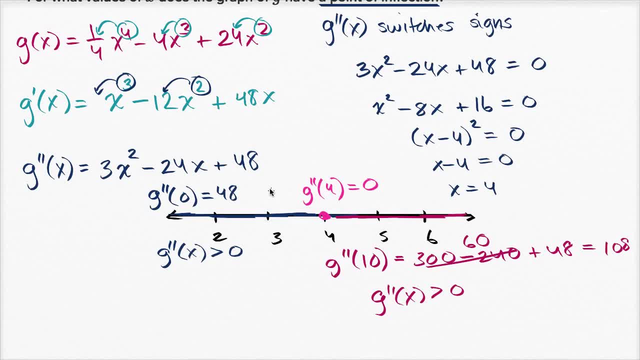 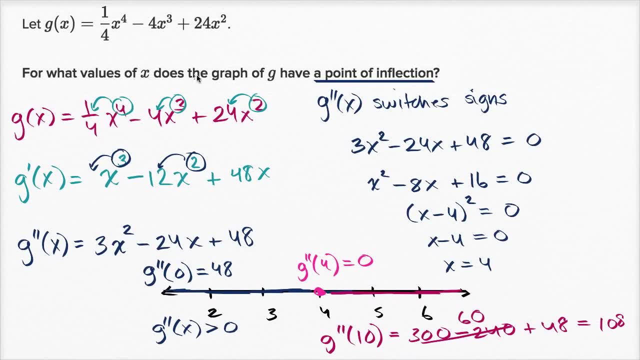 but it's just staying from positive to positive. So the second derivative is positive. it just touches zero right here and then it goes positive again. So going back to the question, for what x values does the graph of g have a point of inflection? 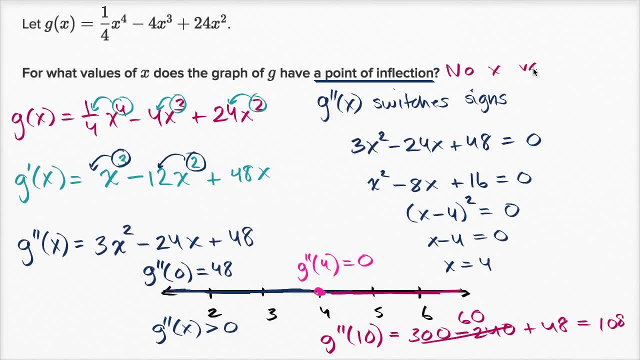 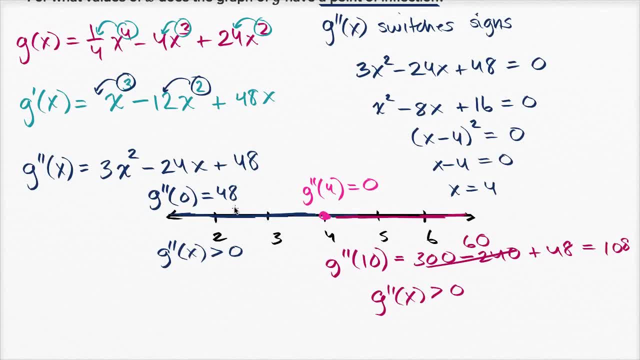 if we switch, if the second derivative switched signs here, If it went from positive to negative or negative to positive, but it's just staying from positive to positive. So the second derivative is positive. It just touches zero right here and then it goes positive again. 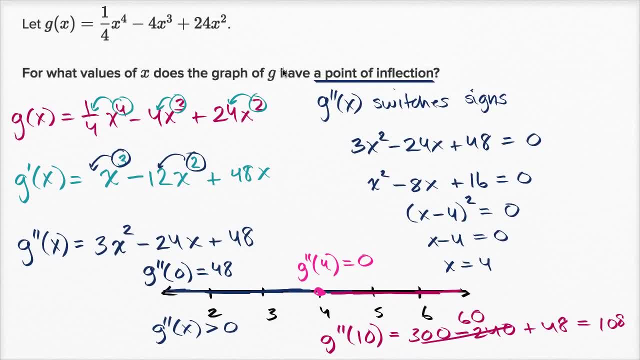 So, going back to the question, for what x values does the graph of g have a point of inflection? No x values. I'll put an exclamation mark there, just for drama.